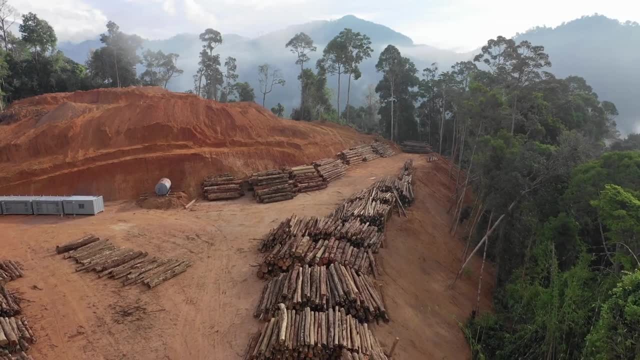 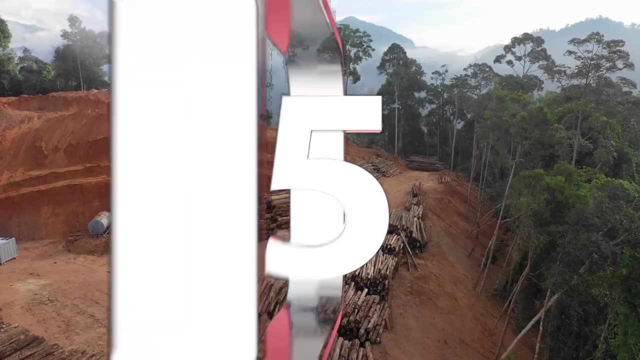 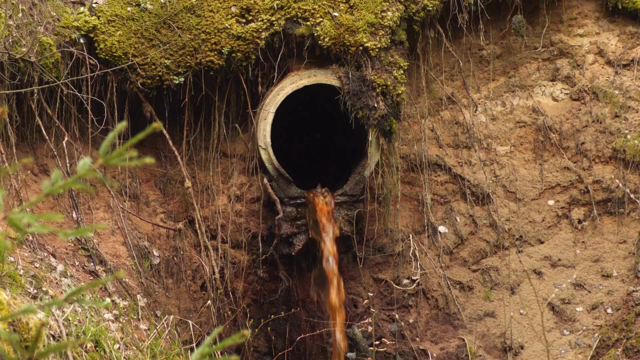 for removing carbon dioxide from the air and providing oxygen. Deforestation can cause soil erosion, desertification and an increase in greenhouse gas emissions. 5. Water pollution. Water pollution occurs when pollutants such as chemicals or waste products are dumped into bodies of water. This can harm aquatic life and make the 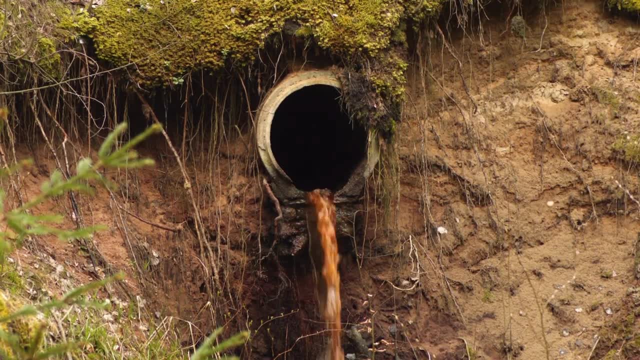 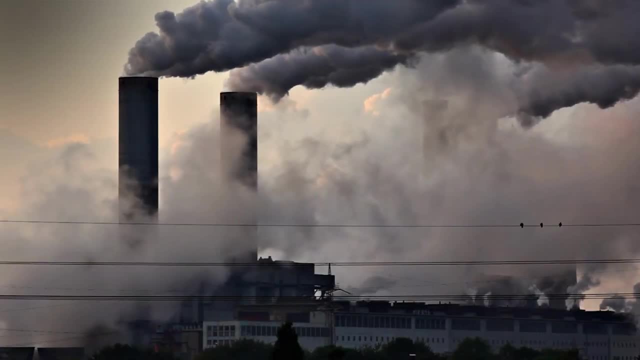 water unfit for human consumption. Polluted water can also lead to health issues such as skin irritation, infections and even cancer. 4. Air pollution. Air pollution is caused by the release of harmful substances into the air. This can cause respiratory issues. 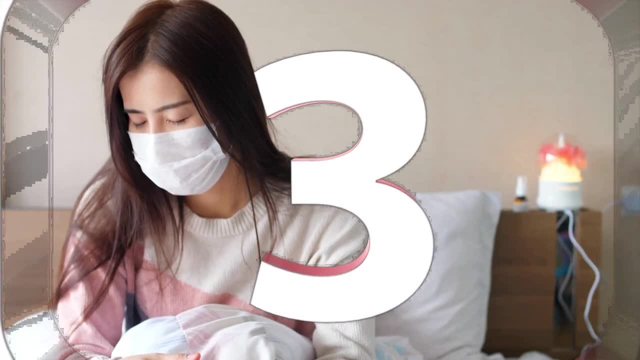 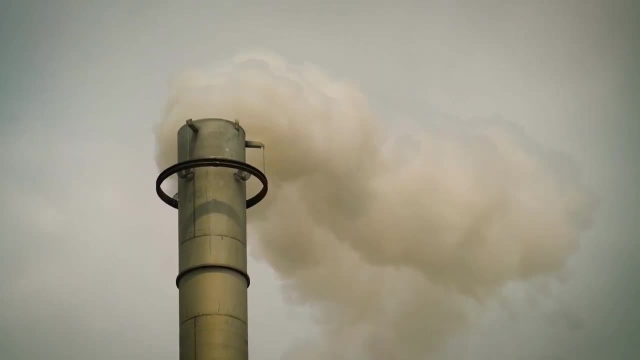 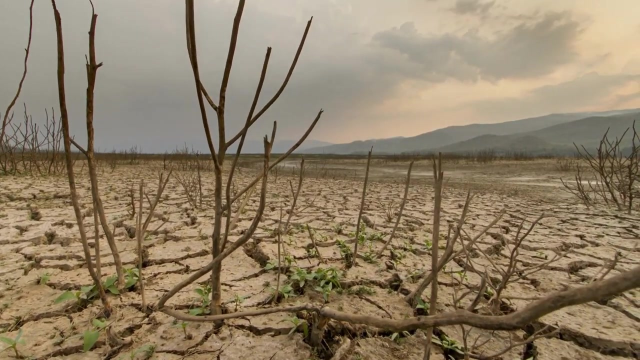 heart disease and even cancer. Air pollution is also a major contributor to climate change. 3. Climate change. Climate change is caused by the release of greenhouse gases such as carbon dioxide and methane into the atmosphere. This causes global temperatures to rise, which can lead to more natural disasters, such as hurricanes. 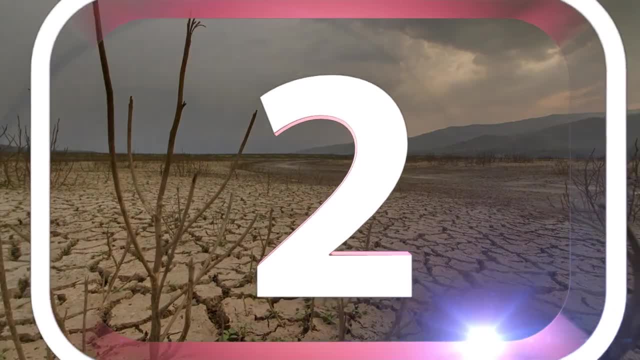 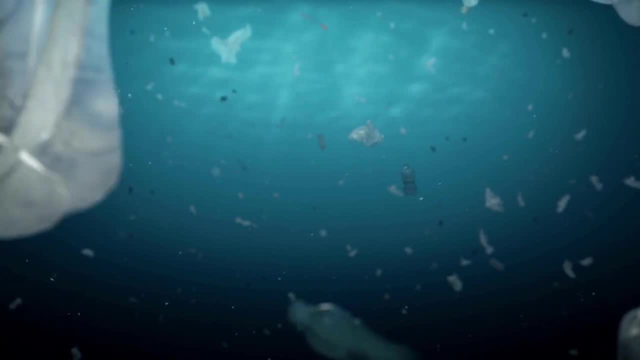 floods and droughts. Climate change also impacts our ecosystems and can cause the extinction of many species. 2. Plastic pollution. Plastic pollution is a major threat to our environment, particularly our oceans. Plastic waste harms marine life and can even make its way into our 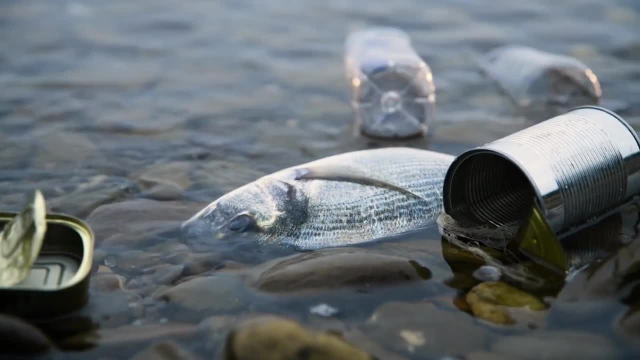 food chain. It takes hundreds of years for plastic to break down, and it can even make its way into our food chain. It takes hundreds of years for plastic to break down, which means it will remain in our environment for generations to come. 1. Loss of biodiversity: This is the biggest. 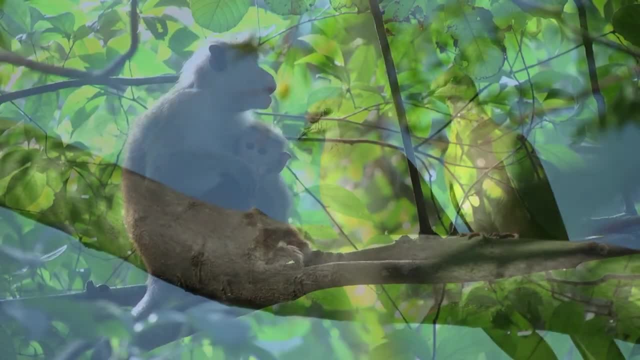 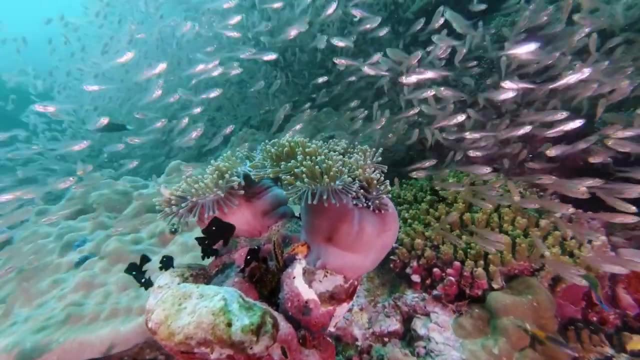 threat to our environment. The loss of biodiversity refers to the decline of the variety of living organisms on our planet. This loss is caused by many of the other threats on this list, such as deforestation, overfishing and pollution. The loss of biodiversity can cause: 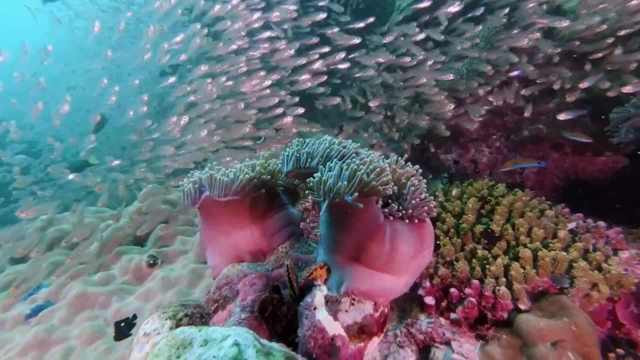 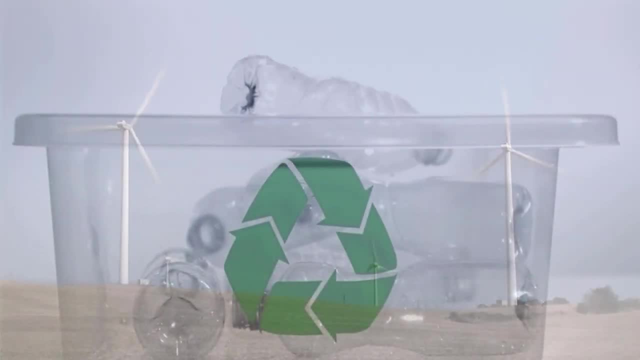 irreparable damage to our planet and can even lead to the extinction of the human race. It's important that we take these environmental issues seriously and work to find a way to find solutions to these problems. We can all play a part in protecting our planet by reducing our 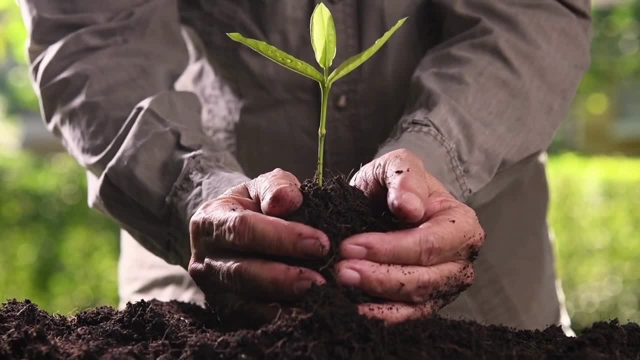 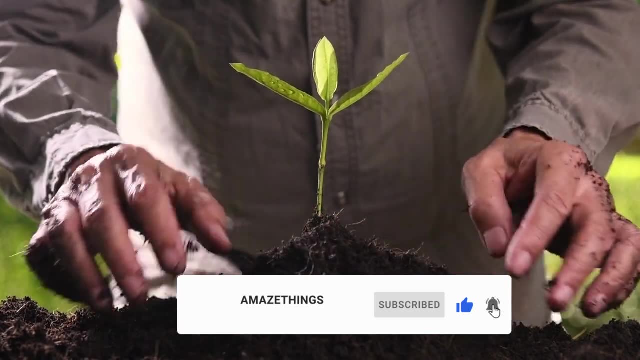 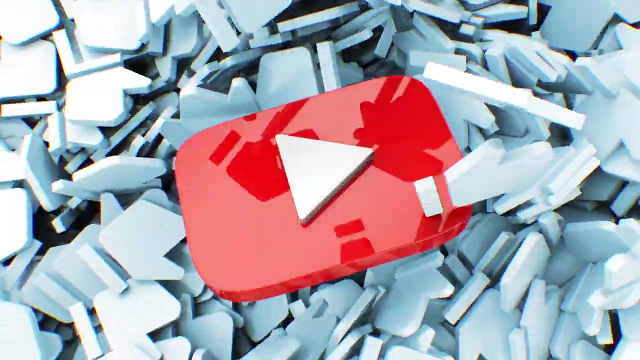 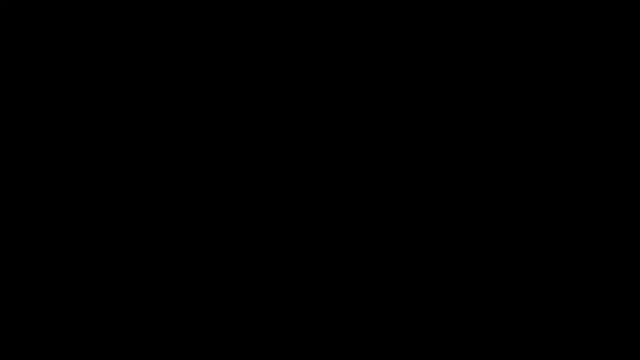 carbon footprint recycling and supporting conservation efforts. Please like this video if you found it interesting and subscribe for new facts every day. Thank you for watching and see you next time on the AmazeThings channel. Stay amazing, you.